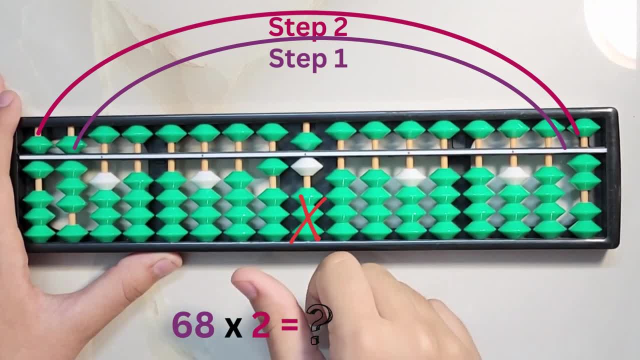 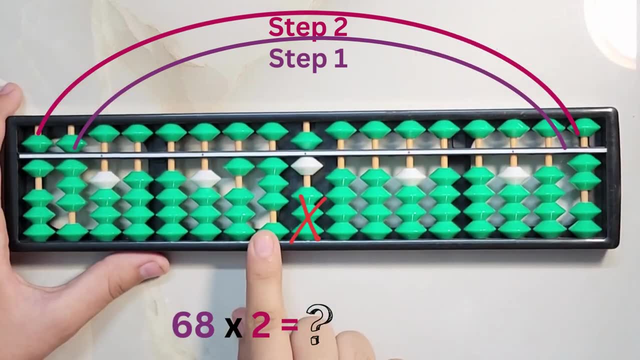 Now this 10's rod is our 1's place, So 2 times 6 is 12.. We need to add here: 2 will be added on the 10's place and 10 will be added on the 100's place. 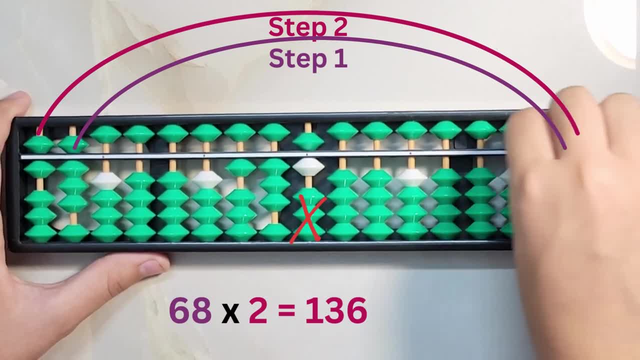 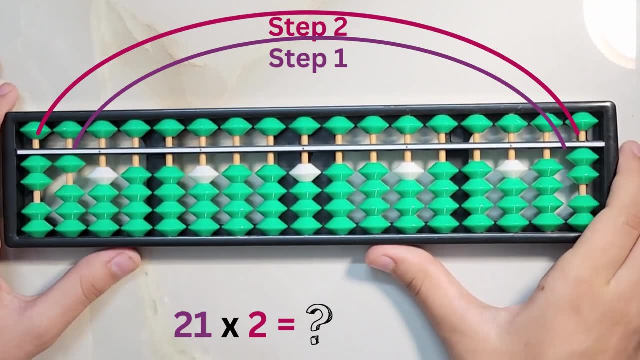 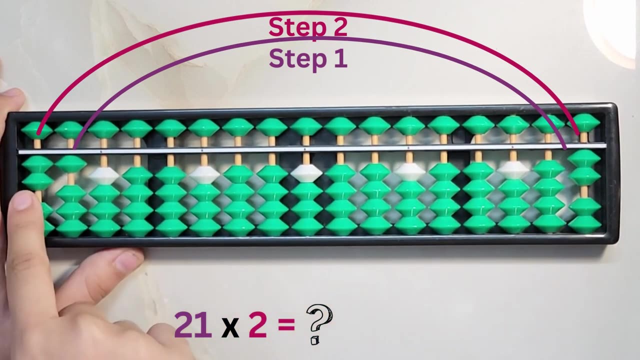 Answer is 136.. 21.. Multiplied by 2. Step 1 is to multiply 2 with the 1, and step 2 is to multiply 2 with 2.. So 2 times 1 gives us 2.. Let's make 2 on the 1's place. 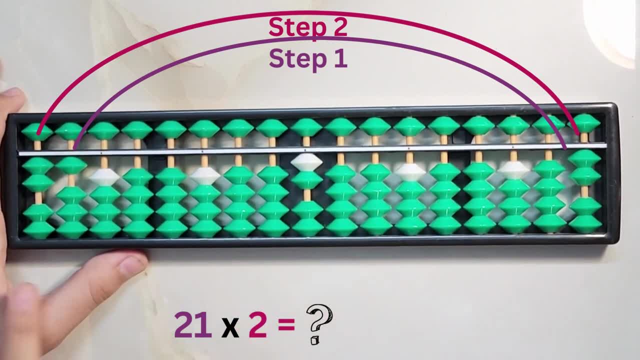 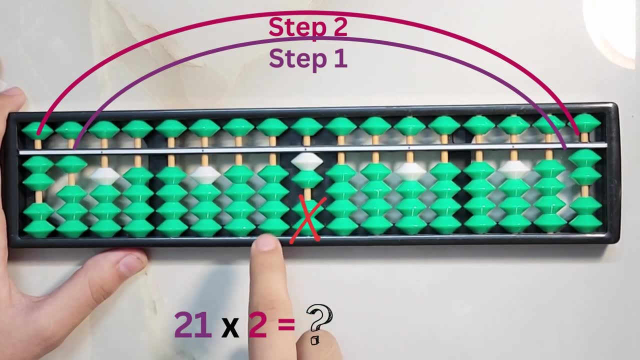 Now that we are jumping from one rod on the left to the other rod, we will also jump from here to here. Remember: now we are standing on the 10's place. Now this is our 1's place and we cannot use this rod. 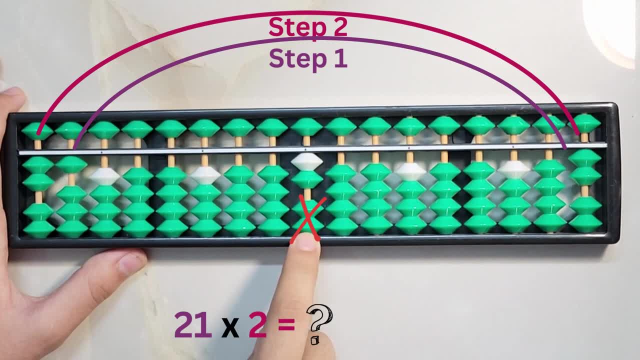 We will use this 1's place again. So the next step is: 2 times 2 is 4.. So we will make 2 times 2 is 4 on the 10's rod, not on the 1's rod. 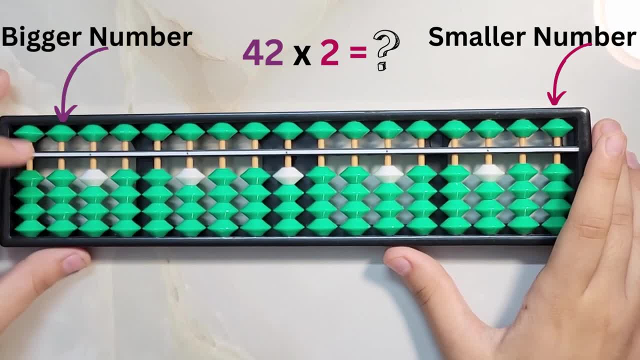 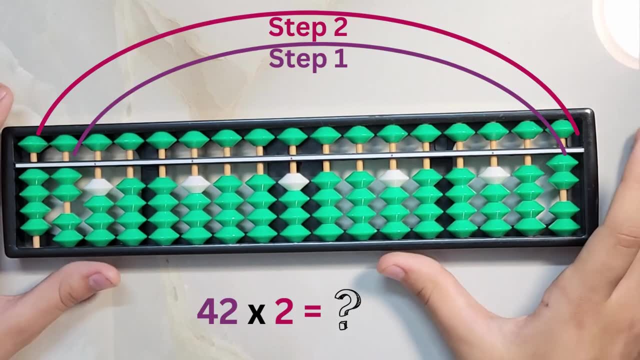 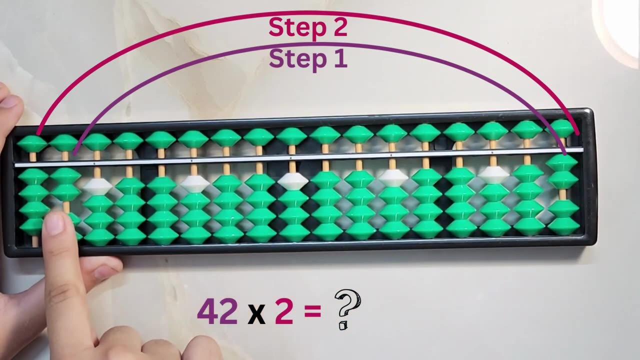 Answer is 42.. 42 multiplied by 2.. Bigger number on the left hand side and the smaller number on the right hand side. Step 1 is to multiply the number on the right with this. Then step 2 is to multiply the number on the right with this. 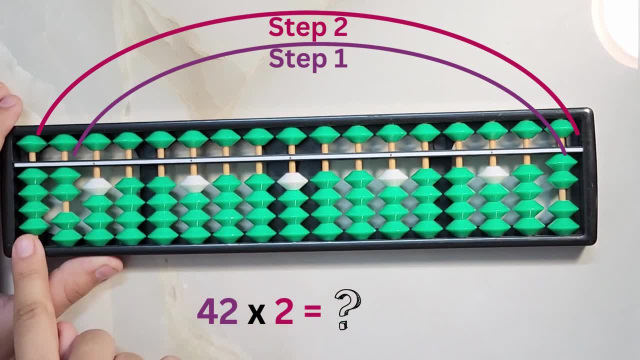 Then step 2 is to multiply the number on the right with this. Then 2 multiplied by 2 is to multiply the number on the right with the next rod. Let's start with step 1.. 2 multiplied by 2 gives you 4.. 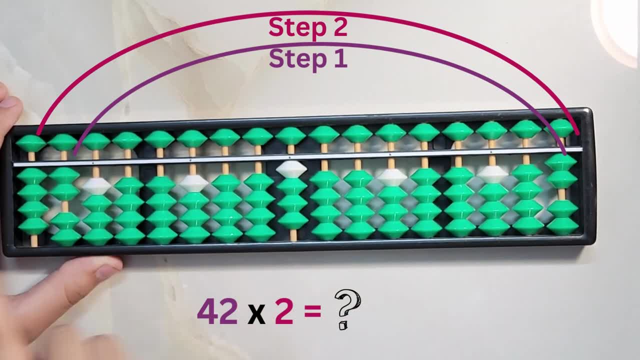 We will make 4 on the 1's place. Remember, now we will move from one rod to another. We are jumping from one rod to another. We will not use this 1's place now. We will also jump here from one rod to another, to the next rod. 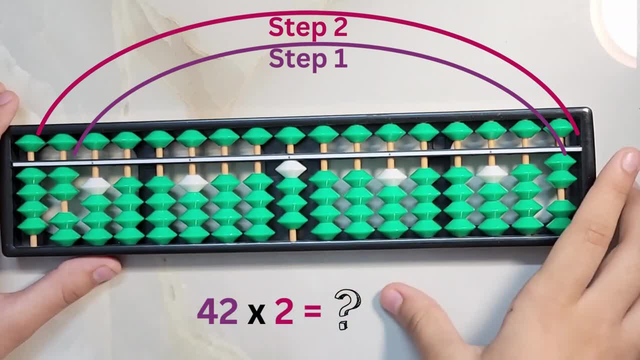 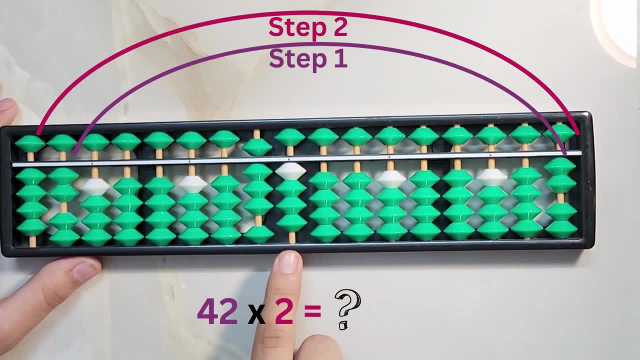 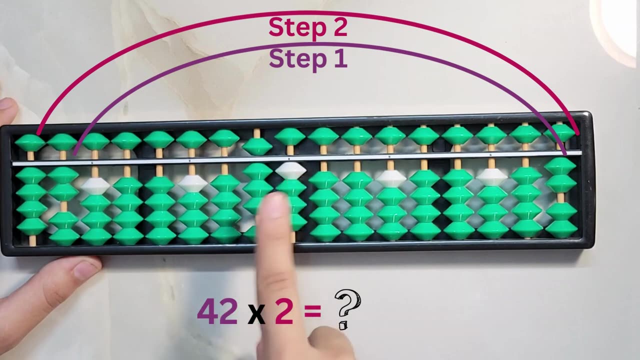 So 2 multiplied by 4, which is 8.. We will make on the next rod, not on the ones place. remember now, this rod is our ones place, this is tens place, and so on. so you cannot use this ones place, which was the original ones place.